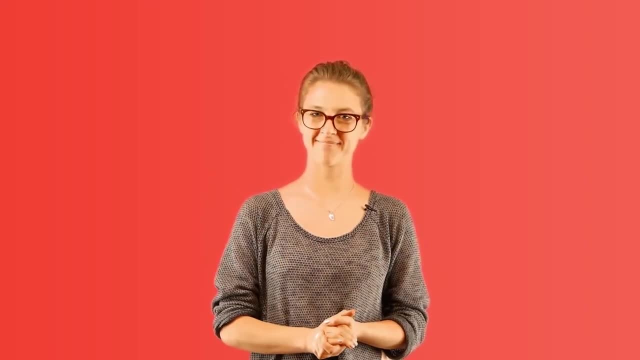 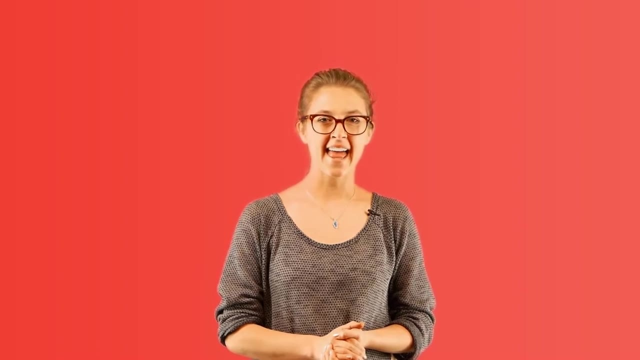 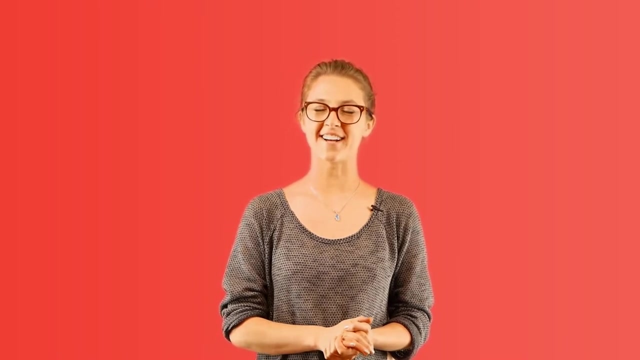 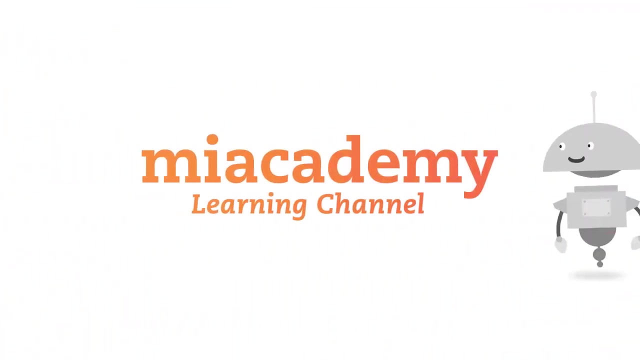 Hello, I'm Kylie and welcome to Beginning Language Arts. Learning more about the English language can be fun. Do you like to listen to stories? Can you learn to read stories on your own as you learn grammar and spelling rules? Let's get started now. 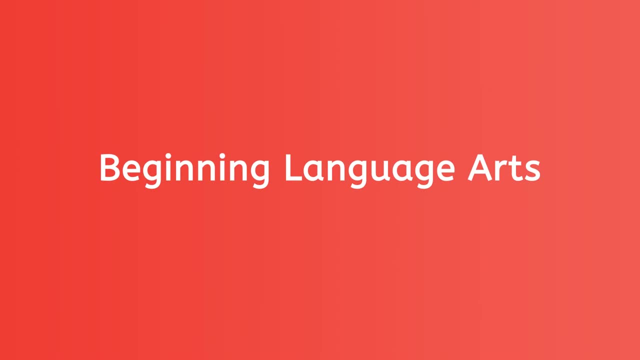 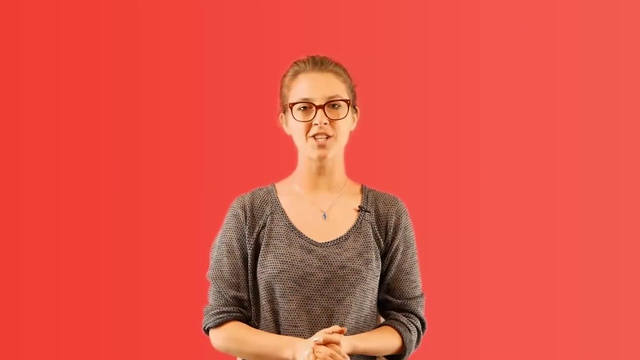 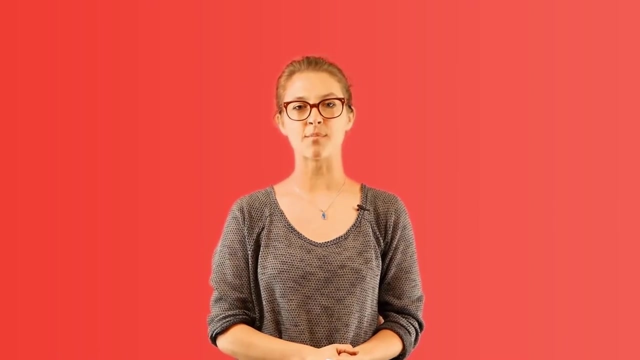 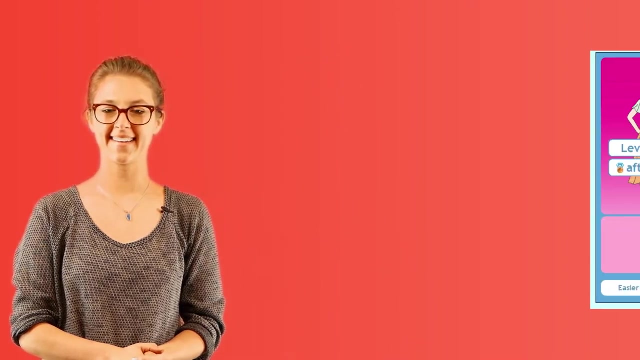 GAME TITLE. In the Beginning Language Arts game, you can expect to practice language skills with fun multiple choice questions. Each of the concepts covered in this game have their own individual videos and games. Be sure to check those out. GAME TITLE. In this game, you will be asked to choose a game. 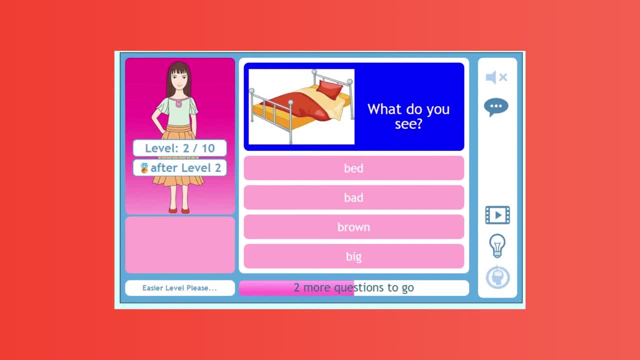 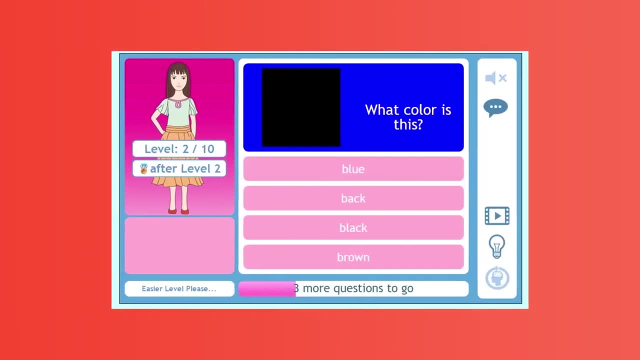 the word for common objects. you see in a picture number words and color words. Be careful: Some of the words in the list are similar, so you'll need to pay special attention to the letters and the sounds they make as you read or listen to each. 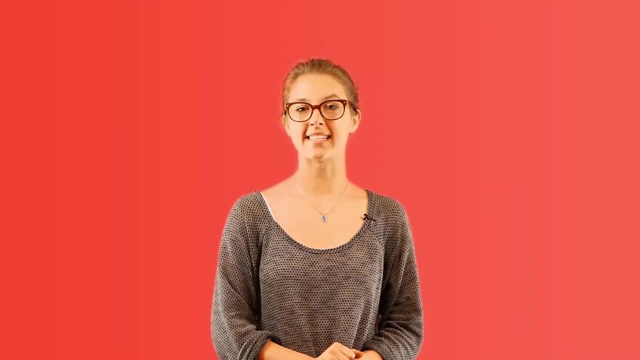 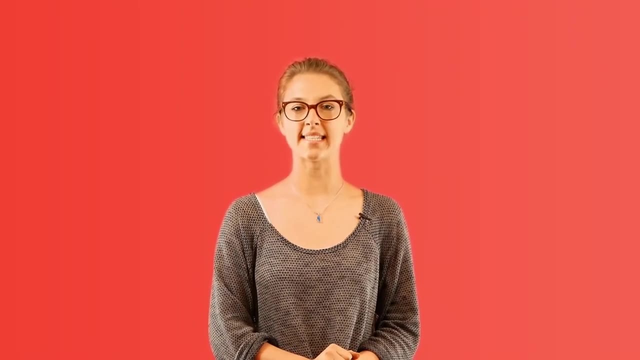 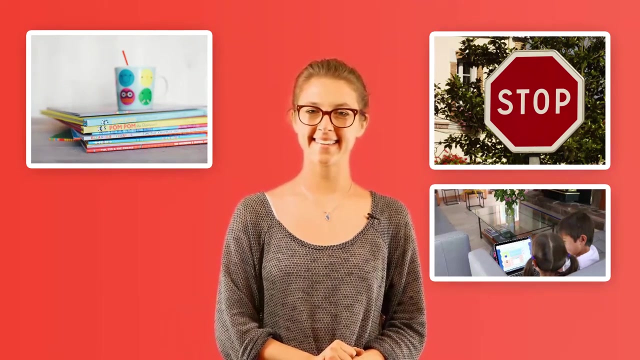 word. This game is a fun way to practice short and common words. Taking this quiz will help you recognize these words in other places, like on street signs, in books or in a tech game. The more you practice, the more you'll improve in. 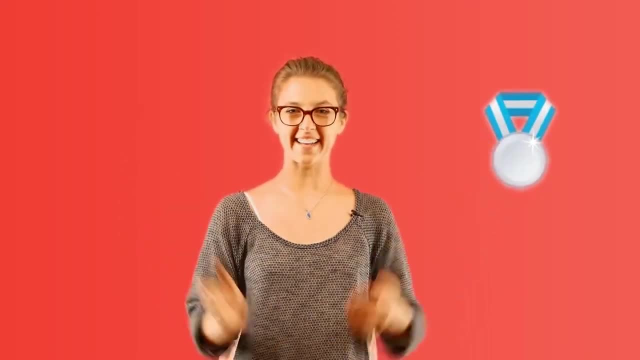 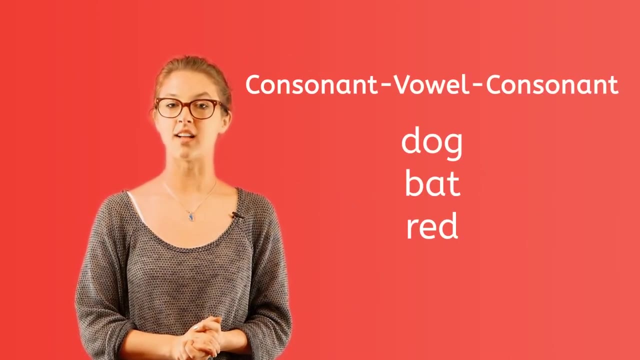 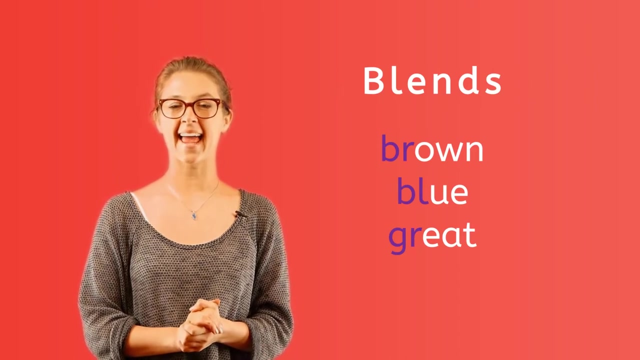 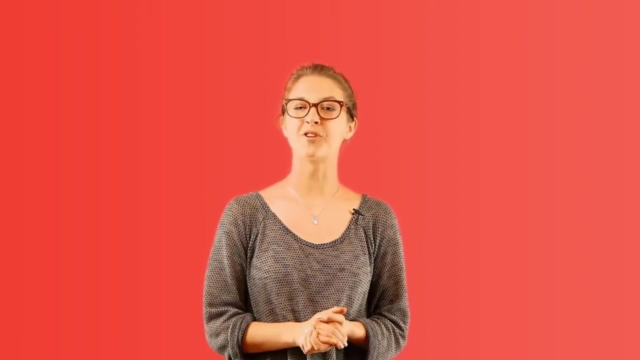 reading fluency And, what's more, you are rewarded. You can expect to practice reading consonant-vowel-consonant words, words with long and short vowel sounds, blends and r-controlled words, and so much more, If you want to boost your reading skills. 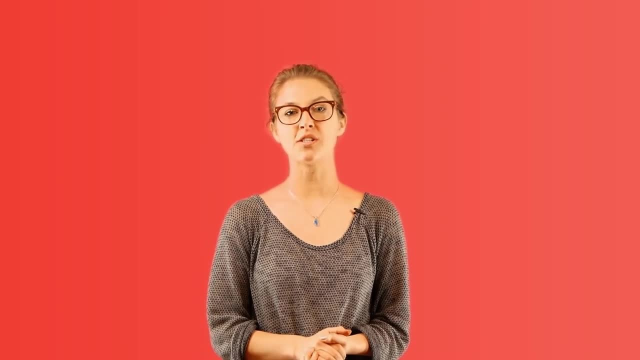 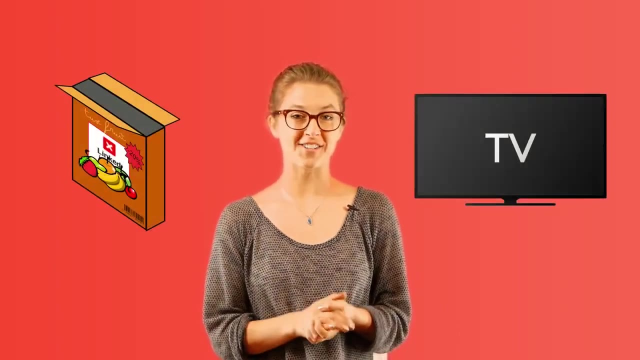 so that you can get better at this game. there are other ways you can do this, both before and after playing. You can read words around your house, read labels at the grocery store or at the grocery store. You can also practice reading words. 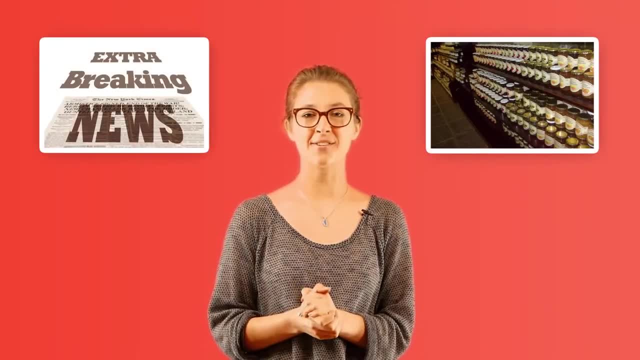 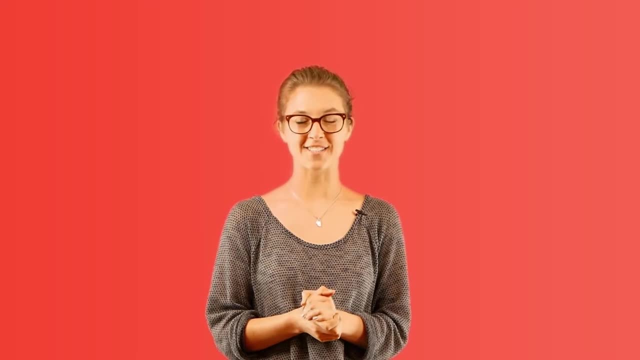 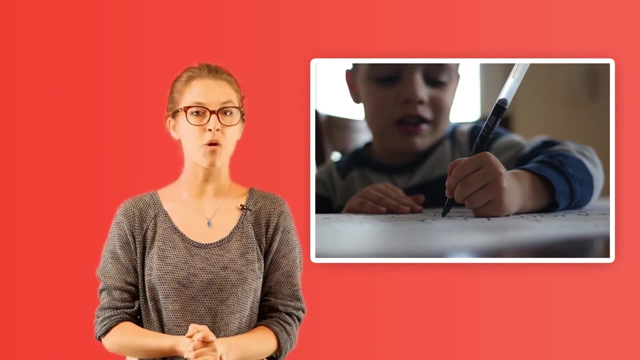 at the grocery store. read headlines in a newspaper, magazine or online. You'll be surprised to find that you can already read many words on your own. You can also practice by writing notes, emails or letters to friends and family. You will